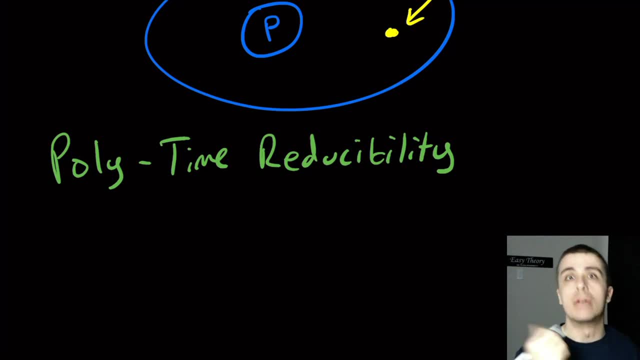 to actually have a restriction on the type of reductions here, which is that they run in polynomial time And the way that we write this is a less than or equal to P, B. So problem: A poly reduces to B, So the P here was M before when we talked about mapping. 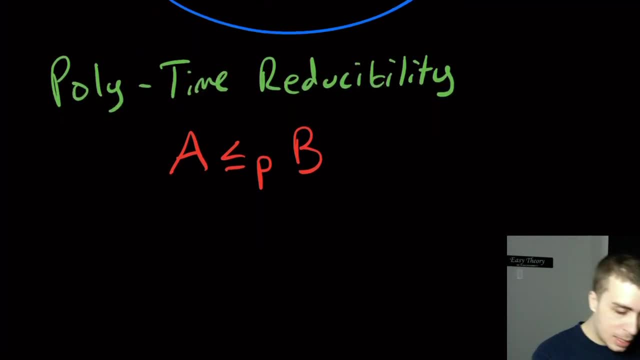 reducibility. Here is polytime reducibility, And what this is saying is that if, and only if, there's some function going from F which is taking strings, not from A, from sigma star, going to, let's say, gamma star, 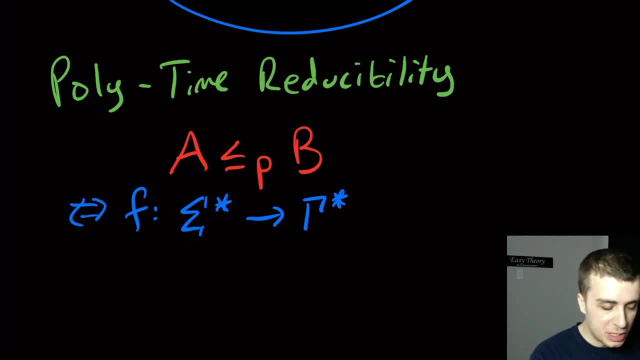 Where A is a language over sigma star and B is a subset of gamma star, Such that we have two different things. We have that F- sorry, We have that a string. W is in A if, and only if, F of W is in B. 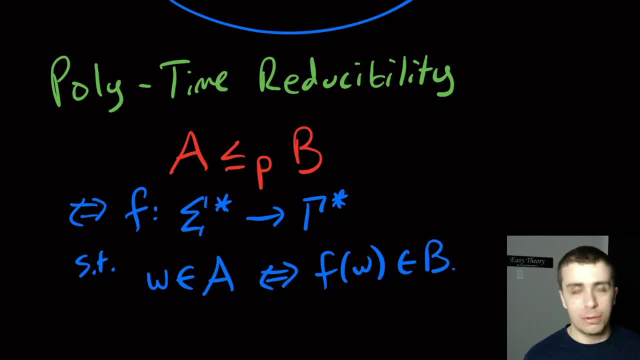 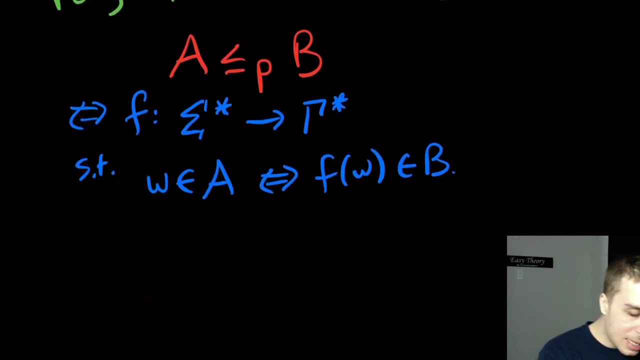 K. so this is the exact same notion as reductions before. The answer of whether the original thing is in A is the same thing as if we compute the thing for b, then it's in b the same time whenever w is in a and what we have is that f runs in poly time. so this isn't exactly right because f is a function. 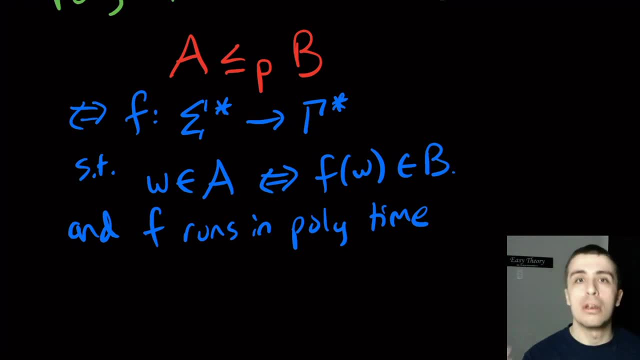 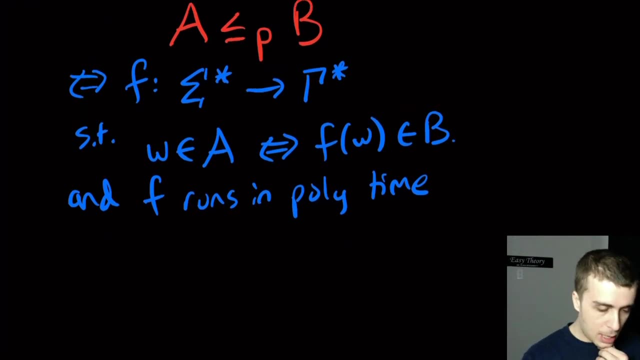 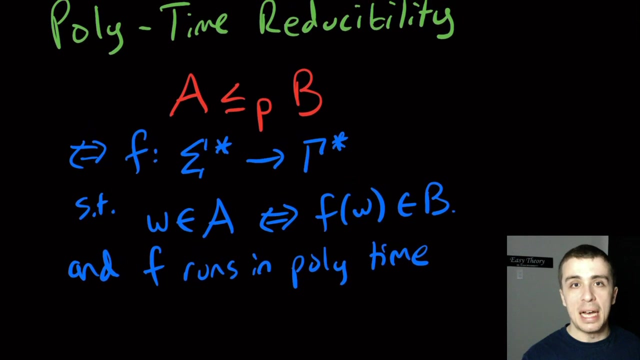 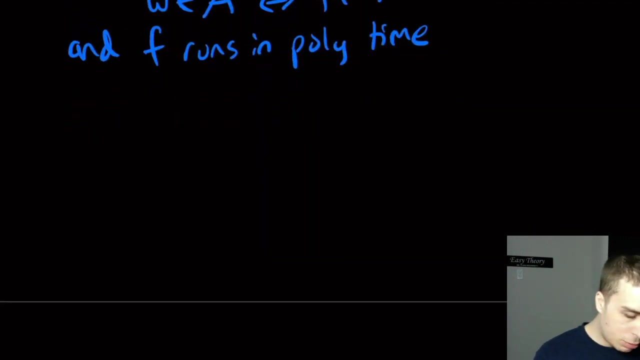 but we mean that we can compute it using a polynomial time Turing machine, deterministic Turing machine, uh, in polynomial time, okay, and that is a notion of reducibility. then a notion of what hardness means is that, uh, we talk about these poly time reductions among np problems. so we're going to say that a language, a, is np hard, if for all. 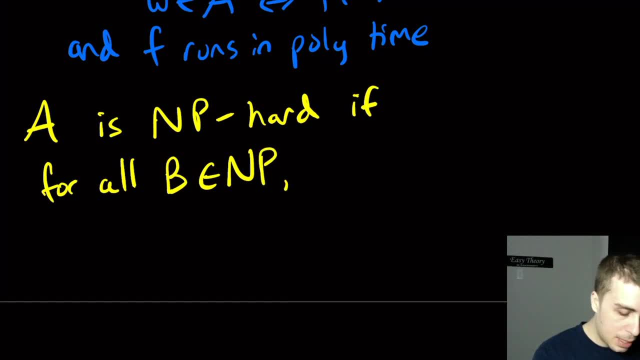 b in np, np we have that a uh. sorry, wrong order, the order really matters here. so b reduces to a. so that means every single uh problem in np, uh poly reduces to a, every single one. um, then we call that problem a, np hard, okay, um, but we're going to make one additional qualification. 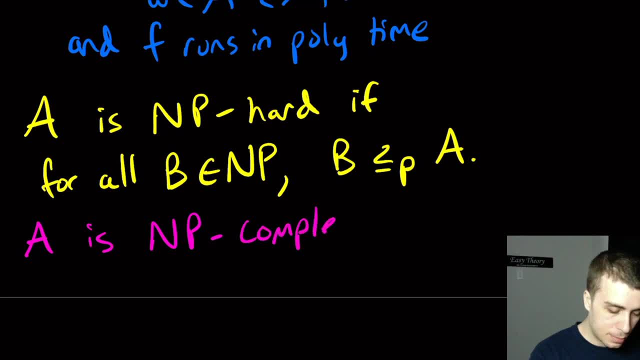 a is np complete. if a is np hard, so that means everything in np reduces to a and a is also in np. so you may think, okay, well, this is kind of silly. well, np hard kind of sounds like you're an np already. it turns out that that's not necessarily true. in fact, atm the undecidable. 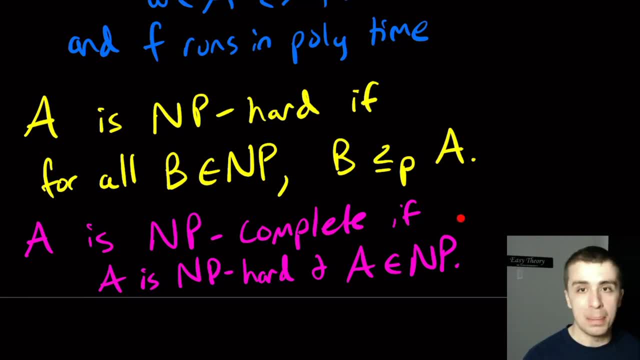 problem is np hard. so that's not necessarily true. in fact, atm the undecidable problem is np hard, but it's not np complete, because it's not in any finite time language class and certainly np is not in there. so we want to talk about np complete, because those are the problems. 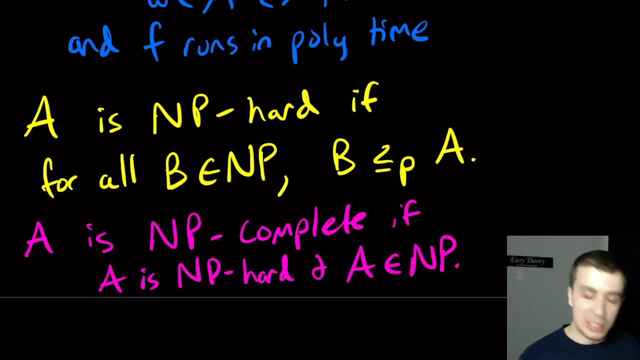 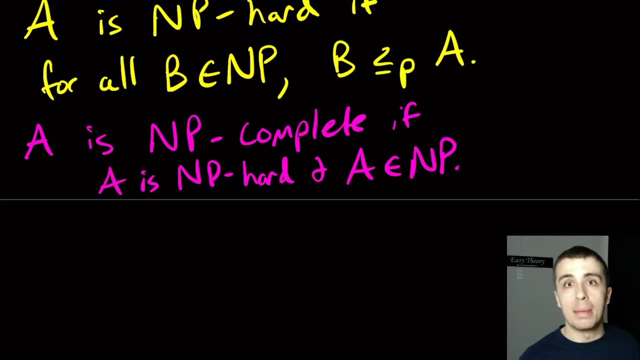 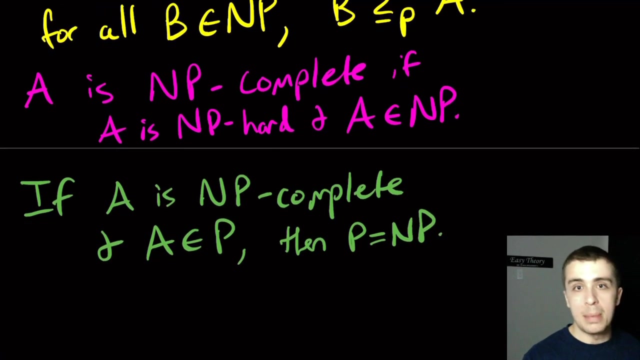 in np but are the hardest ones, because one thing that we can find out is: well, if any np complete problem is in p, then p equals mp. so if any, let's say, a is np complete and a is np, then p equals mp. so i'm not going to formally prove this, but why is this true? so np complete means obviously. 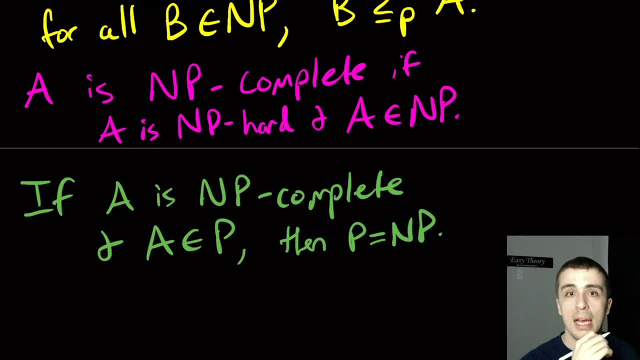 everything in np poly reduces to uh a. so then what we can do is: okay, well, a can be run in polynomial time. so take the. the second式 to be ruled out: you can't lump np together into an academic fault. you have to make it work. oh, yeah, okay. so the second one is: if you take a plug and then you split the two cour, excuse me, in a minute you can't mark up the pickup point. that's nothing you can seek. 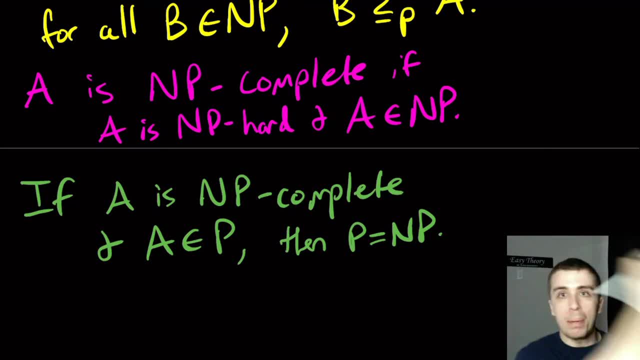 let's see what happens. something is found out here in this example. I'll make another example. whatever input for B you got, do the poly time reduction to a, so then the resulting instance for a is only polynomially larger, because the whole reduction takes polynomial time. and then compute the thing on a or with some. 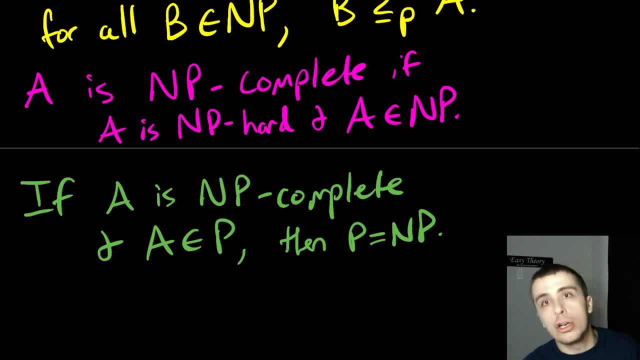 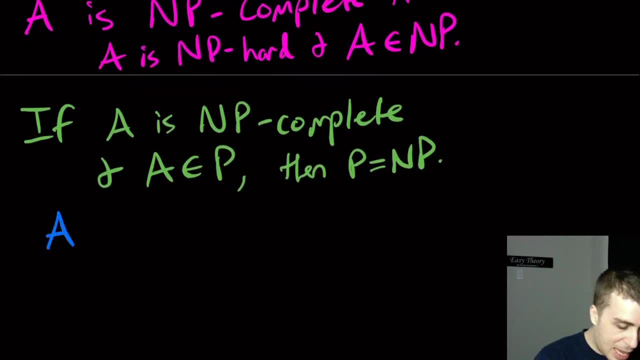 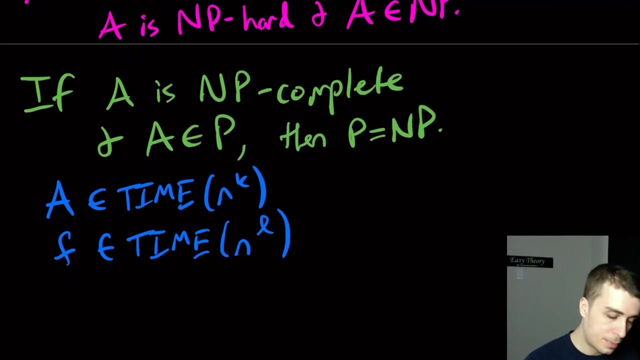 poly time algorithm for a and then the answer corresponds to that of B. well, let's actually figure that out. so let's say that a is in time N to the K and the compute, the function itself, is in time n to the L. let's say then, doing the 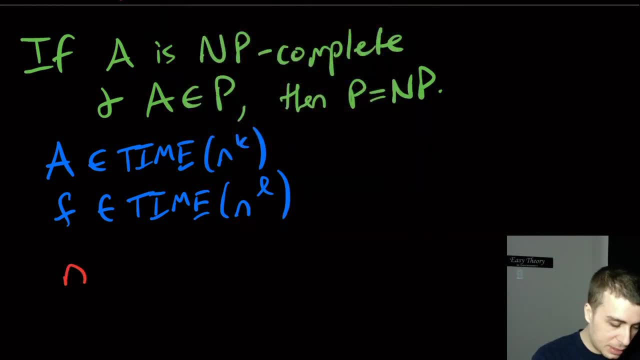 reduction will. we'll see. so if we have an instance of size n, then the reduction F will, an instance of its size, will get us an instance of size Zs instead. let's say that element minus, so we have an instance of size Z. our instruction: if we 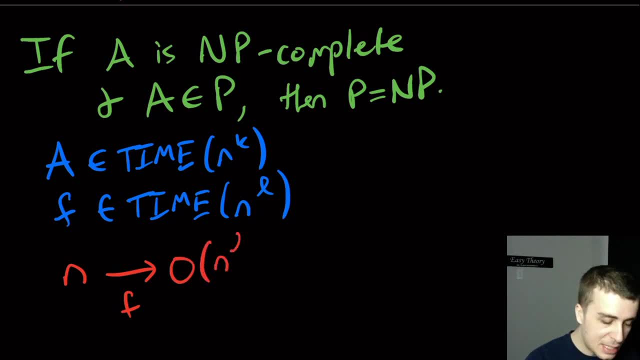 of size at most n to the L. so I put a big O here because it could be less. but then running the algorithm for a will take an input of this size to the cave power, and so then the running time for a would be at most n to the L to the power. 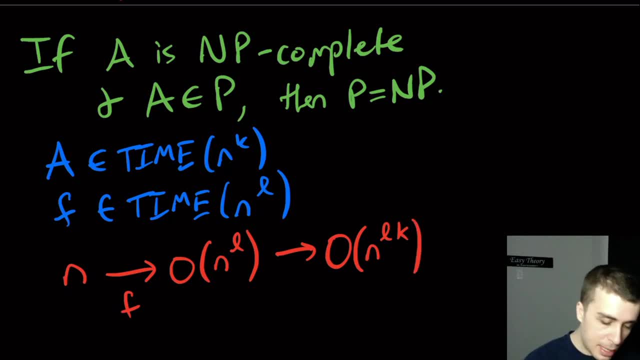 K, which is L, times K, upstairs and notice that this is still a polynomial because it's just a number times another number. so here is the algorithm for a, and so therefore we have shown that the, so this is a, the running time for the algorithm for B, and so B runs in polynomial time, and since every problem in NP reduced to 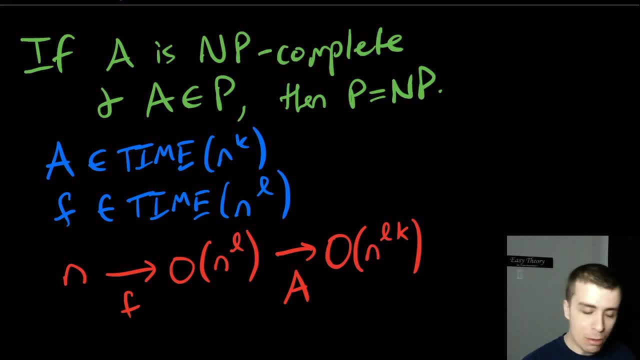 a, then that means that every single algorithm will take this a polynomial amount of time for every problem in NP, and so therefore we have concluded that if a is NP complete and it's also in P, then these are the are the same, the P and NP are the same, so that would imply that a is: 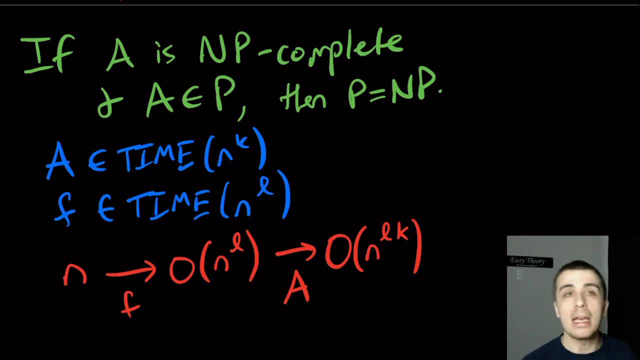 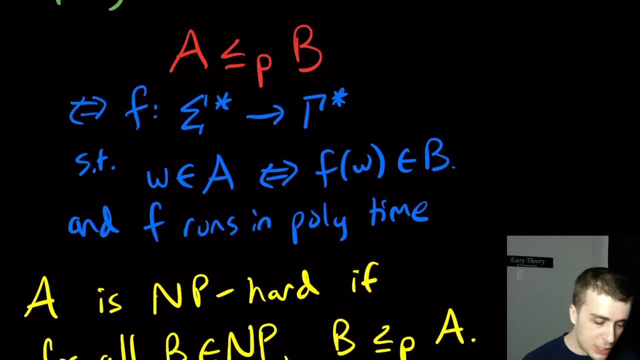 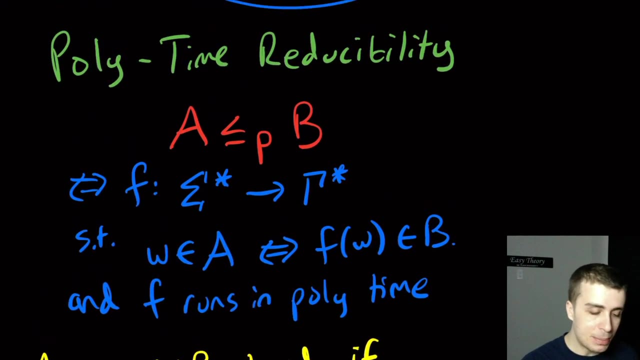 sunk, in some sense, the hardest problem in NP, because if it were in P, then P and NP would be the same, and so I shouldn't mention one thing, which is that poly time reducibility is the one that's usually used, but sometimes we would want to have a more strict notion of reducibility, so sometimes we restrict. 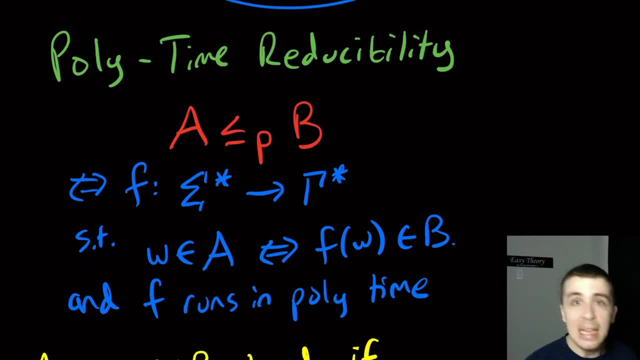 here to say not any polynomial, but maybe linear time reduction or maybe logarithmic space reduction or something that's more constrained than polynomial time. but here we're going to use polynomial time because that's what everyone used for a very, very long time and it's what everyone is used to. so 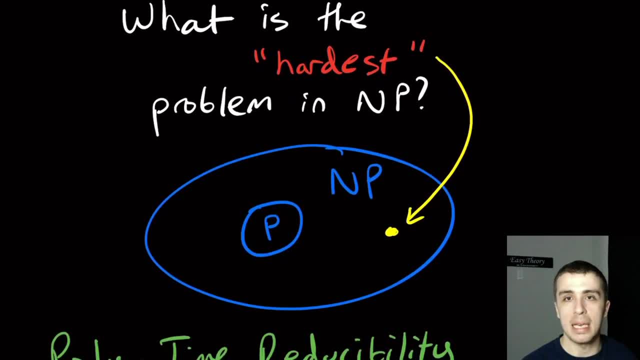 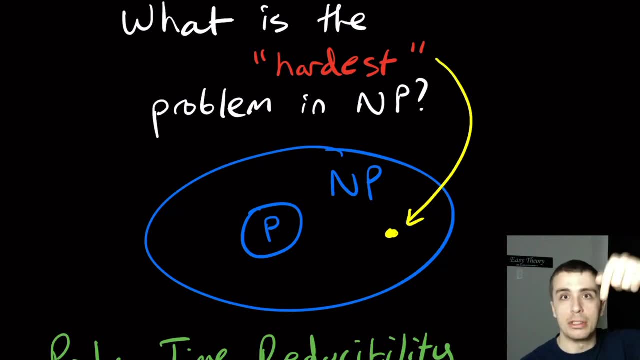 hopefully that was interesting. leave comments about P versus NP in the comments down below. as always, please like the video and subscribe to the channel. really helps us out. there are many other links in the video description if you want to support the channel further. and, as always, thanks for watching and I'll see you next time.